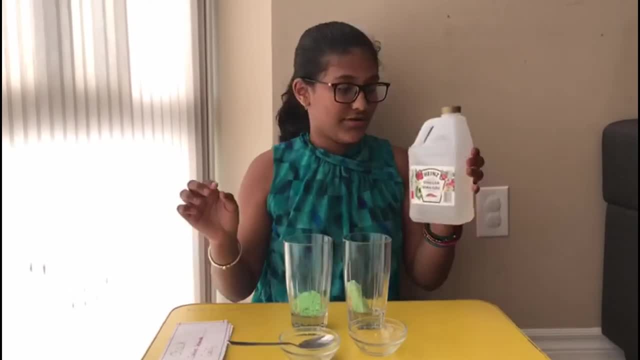 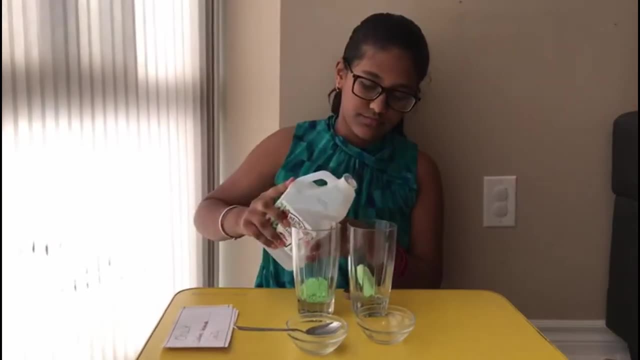 Pretty easy and straightforward. right Now, let's add the vinegar. I'm going to add a little bit of water and mix it. I'm going to add a little bit of salt and I'm going to add a little bit of vinegar. 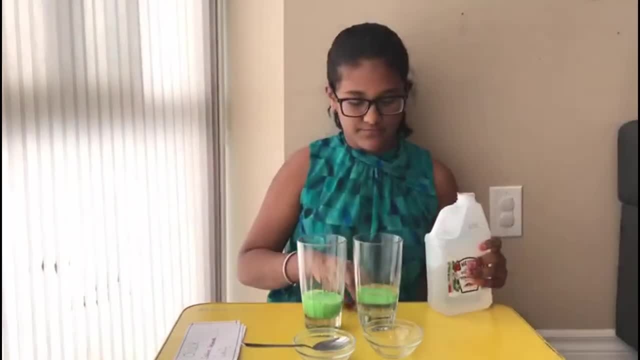 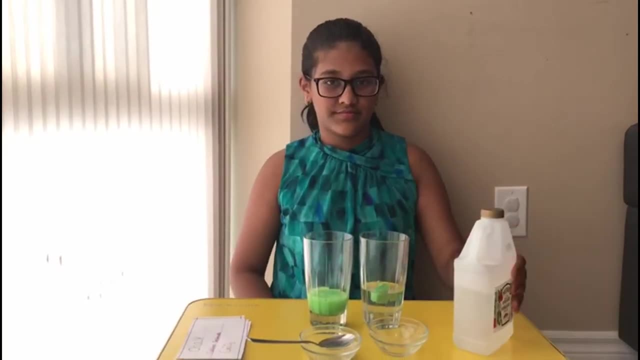 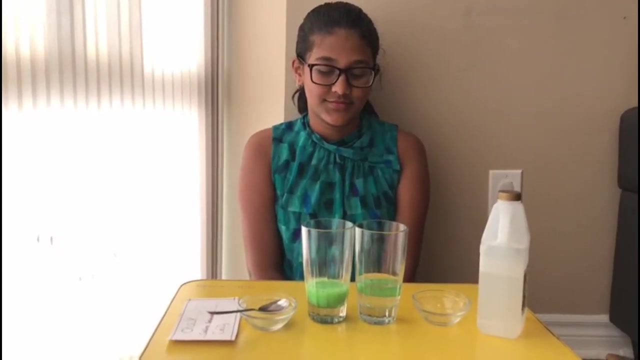 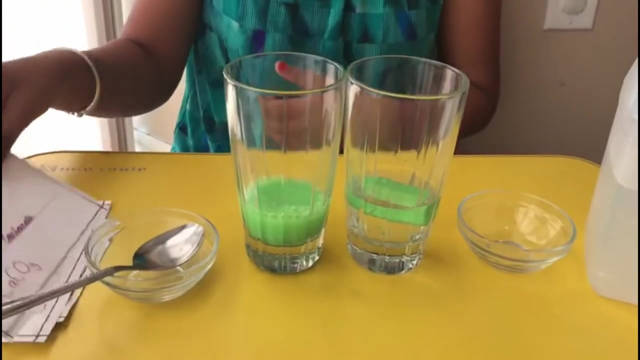 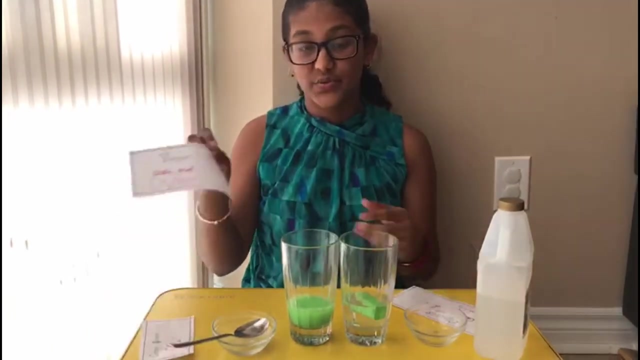 I'm going to add a little bit of vinegar and I'm going to add a little bit of water. Now I add the vinegar. Now observe. What do you think has happened? I think the vinegar is completely gone. Chalk contains calcium carbonate, CaCO3, which reacts with vinegar. acetic acid CH3COOH. 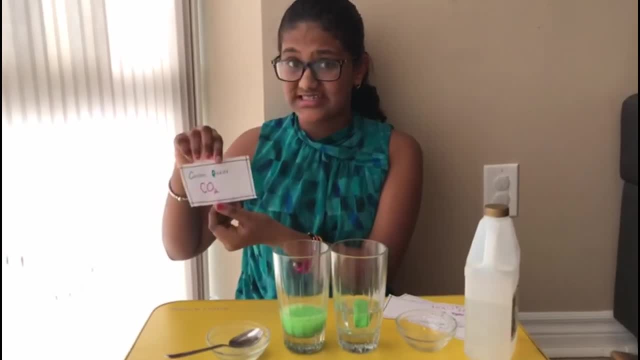 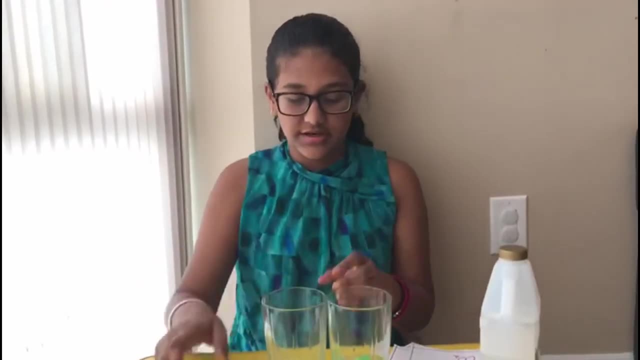 and at the end it forms a gas called carbon dioxide, CO2.. Some of the mass of the chalk is lost to form this gas, making it smaller. For example, if you see this one, this is the one where I put the crumbs. 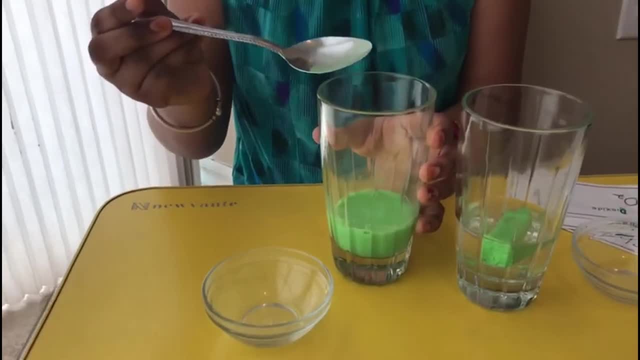 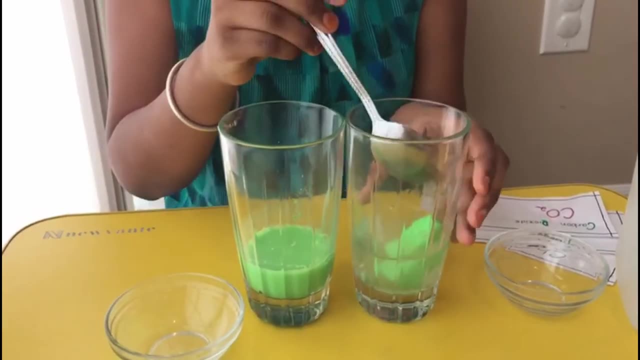 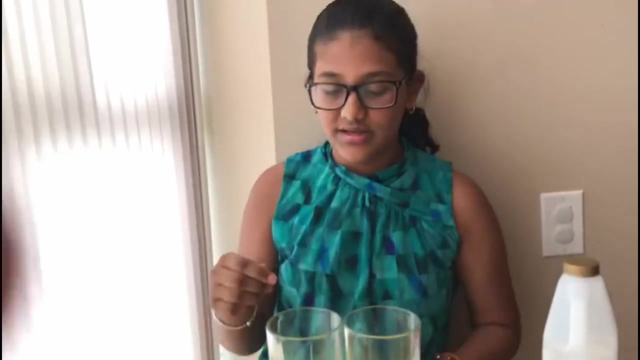 And it's almost all dissolving, But while this one, this one is still in a solid shape, so I think it's going to take more time. As you can see the one, the chalk where I smashed it, and there were, I put the crumbs. 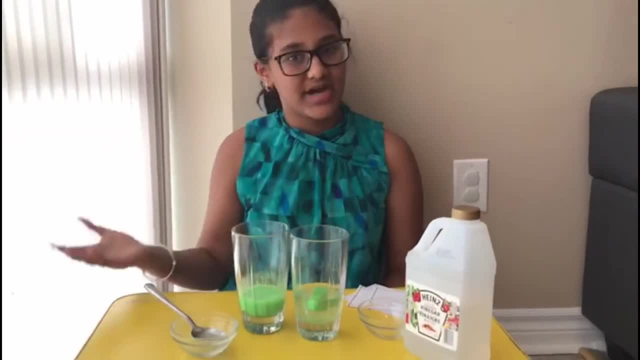 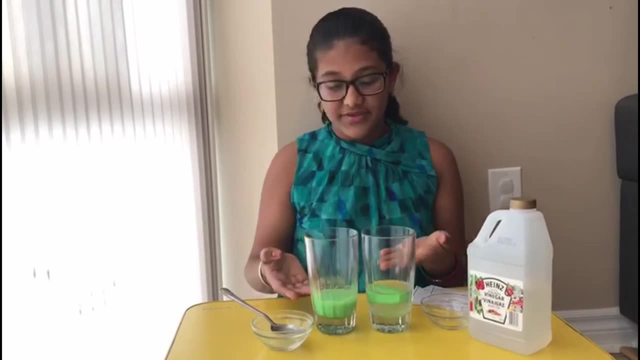 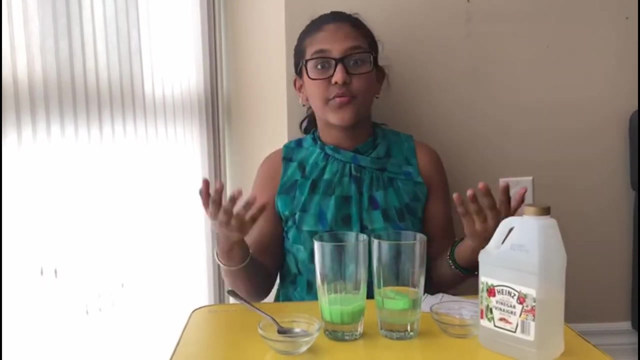 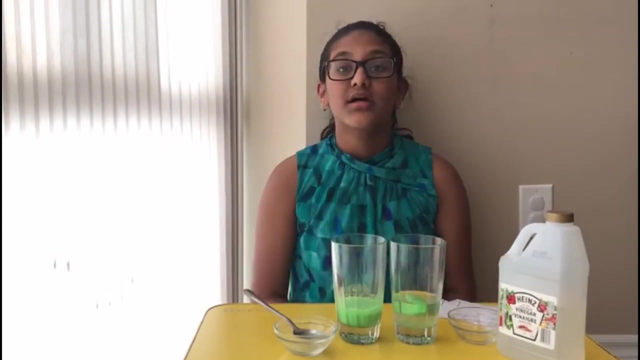 in They were. that reaction happened much quicker, while the solid one is still taking some time. You can actually see these because first, when I poured vinegar into this container, this glass, more bubbles popped up, So that means more carbon dioxide was actually pushing up. 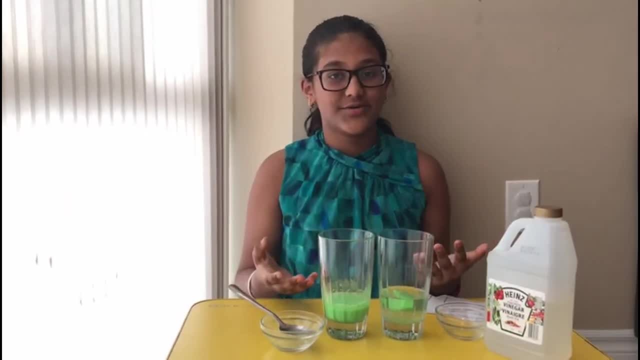 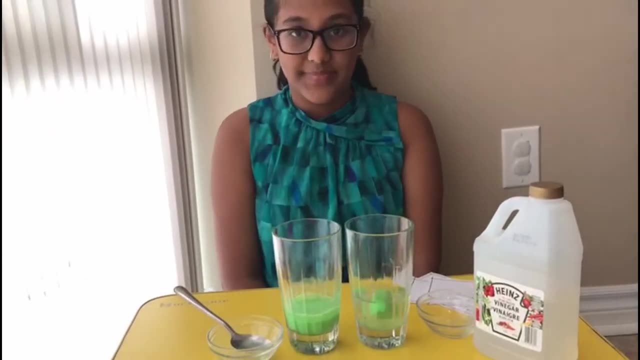 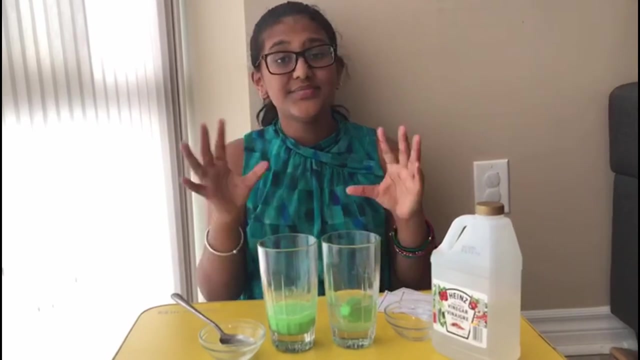 When the chalk is broken up, more surface area created on the small pieces for the reaction to occur. The same thing happens in nature, But instead of chalk and vinegar, limestone and acetic rain is used. When limestone is in smaller pieces, it dissolves more quickly, like here.